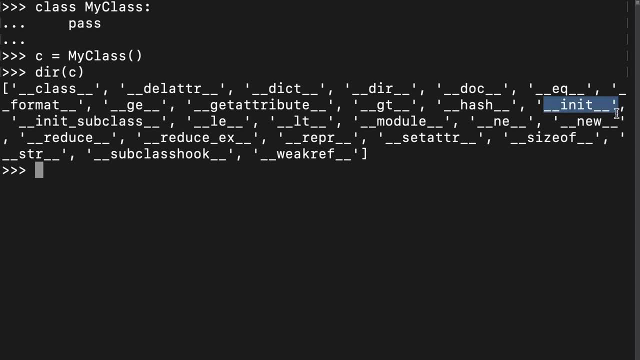 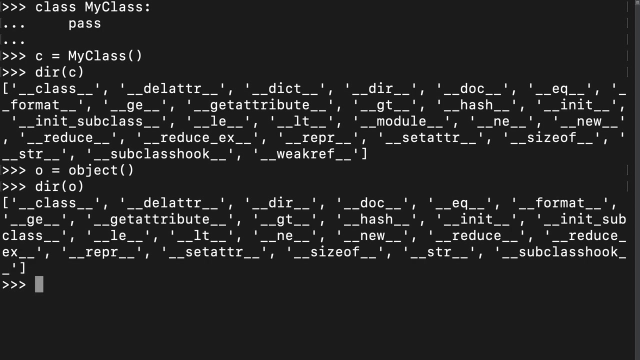 may look familiar to you, Such as dunder init, which we use as the constructor for constructing new classes. We also used init to declare instance attributes. To explain where these are coming from, let me create one more object and list its members. And would you look at that? It looks like the. 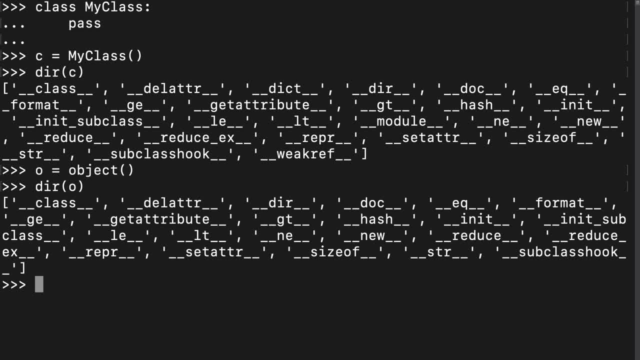 o object and the c object have very similar members, Except the c object has very similar members. The c object, which came from our custom class, has some extra members like dunder weak graph. You might be able to guess what's going on here, but let me explain This o. 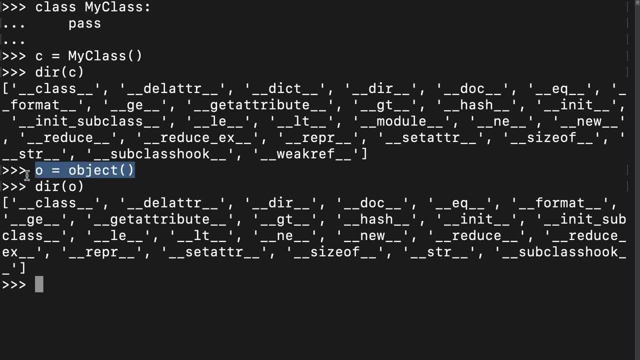 object was instantiated from the object class, which is super confusing, considering we've been calling every instance of any class an object. Well, this object class is not a class that we define ourselves. It's built into python and it's this object class that defines the strange members And, as it turns out, every 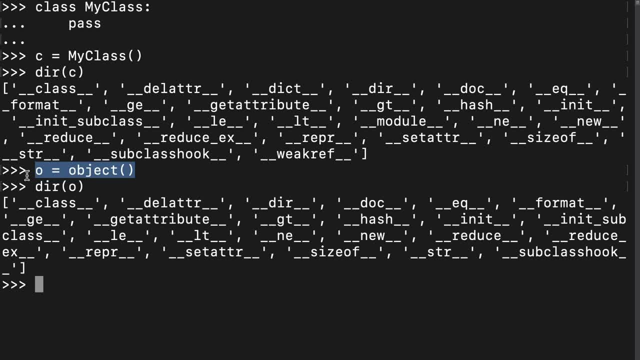 custom class that we create automatically inherits from this object class behind the scenes, even if we don't explicitly make it. That explains why the c object has all these members too. It inherited it from the object class. The extra members present in our custom class came from the different members. By this we mean that the c object inherited. 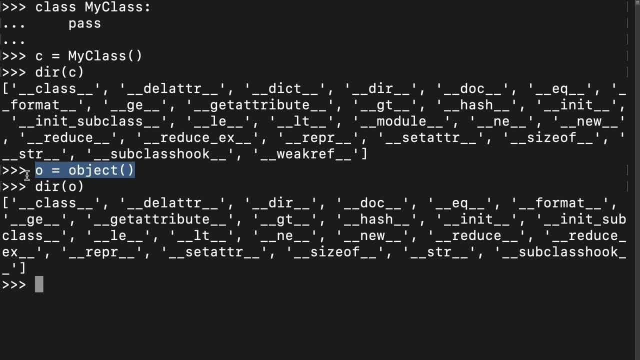 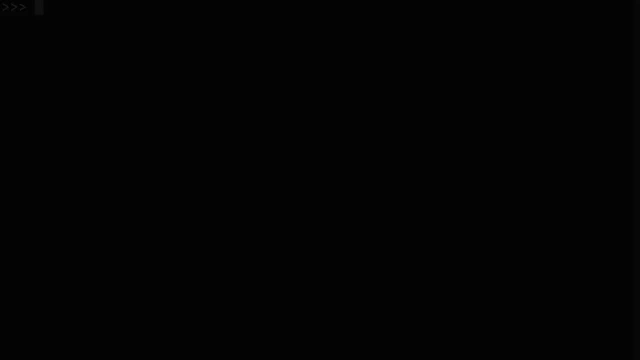 from the object class, And we can see that the dunder weak graph, though, contains these from elsewhere, but that's beyond the scope of this course. The point is, every class in Python implicitly inherits from this object superclass, which defines all these magic methods that Python uses to manage our objects. 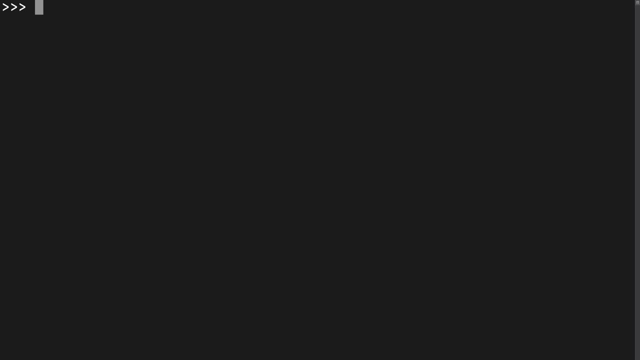 Another place where inheritance is used is with exceptions. Exception objects are special in that they can be thrown up a call stack and caught anywhere along that stack. If no code catches that exception object before it reaches the top, the program crashes and you're left with a stack trace. 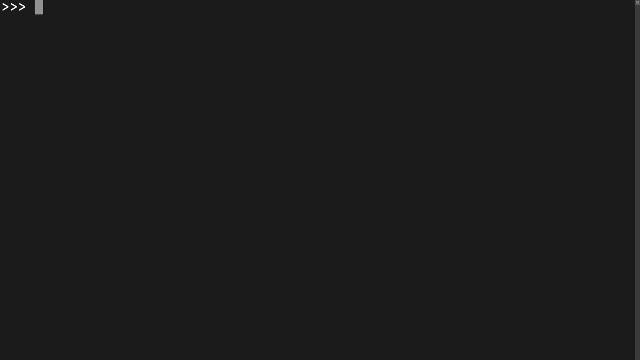 If you're interested in learning more about exceptions, we have a course for that, which I will link down in the video notes below. Let's see how they work with inheritance. Someone new to exceptions might try to create their own exception class as if it were a. 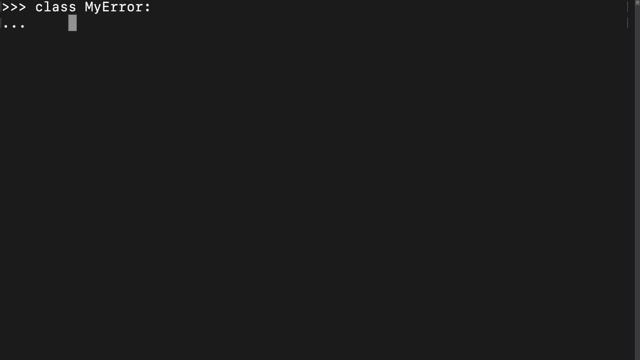 normal class, Just like this. Exceptions can be raised with the raise keyword. This is similar to throw in other languages. Alright, we got a stack trace, but it's not from our exception. There's a type error, not my error. 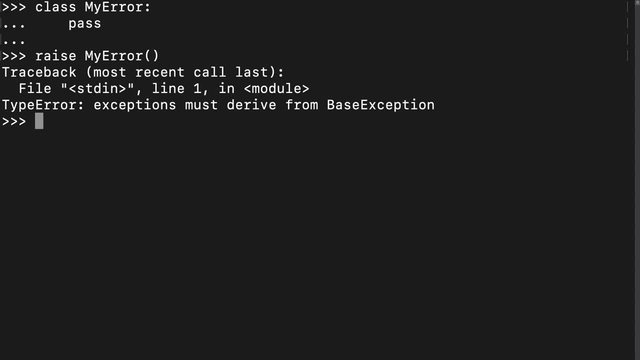 Python has identified that we're trying to create a custom exception class, but we didn't do it right. It's saying that our class must inherit from our exception class. We can use that as a reference to the base exception. Base exception is a built-in class provided for all error types. 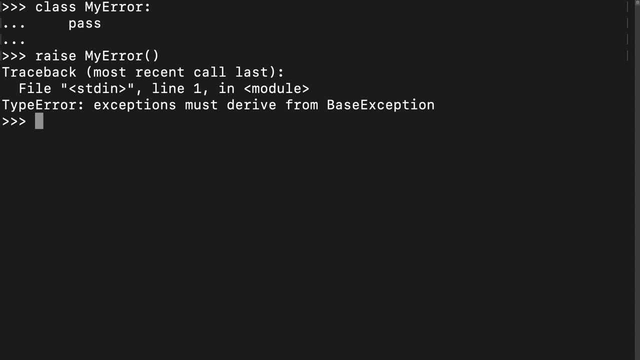 There are lots of classes that derive from base exception, such as syntax error and arithmetic error, which means that we can use them in place of base exception. Remember, if syntax error inherits from base exception, it means syntax error is a base exception because it inherits all of the members of base exception. 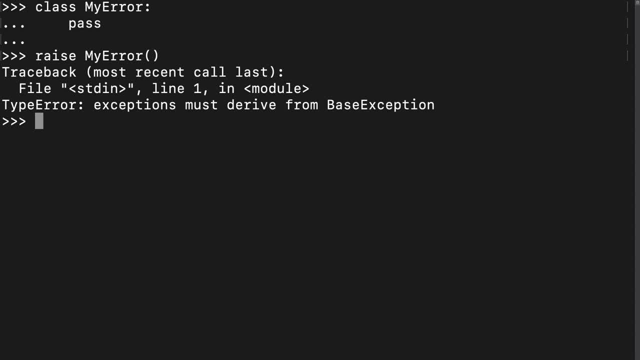 What specific exception type you inherit from depends on the situation at hand. Base exception is not supposed to be inherited from directly, so we'll choose its next child a class called exception. This is the class that the official documentation recommends inheriting from. 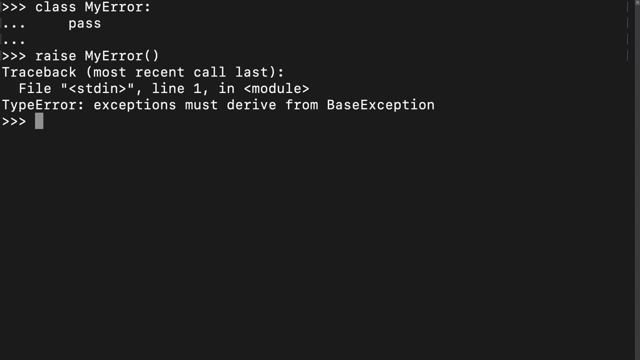 I'll redefine the myError class, But this time I'll put the name of the class I want to inherit from in parentheses after the class name. My error is now an exception. literally I could write pass in here and leave the custom exception type blank. but I want to do one. 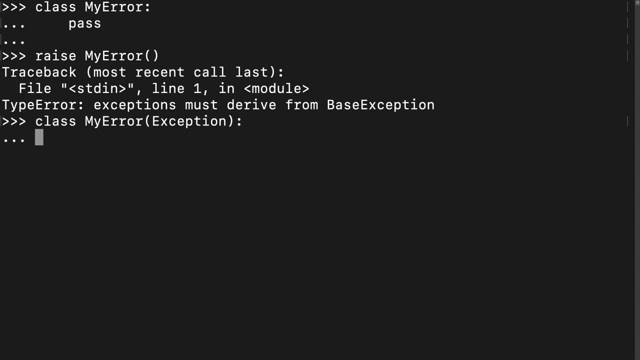 more thing, Exceptions usually have some sort of message that's intended to tell the user or developer what went wrong. The exception class contains an attribute for the message and as such, it's been passed down to our myError class. To use it, we first must add an init method to this class.